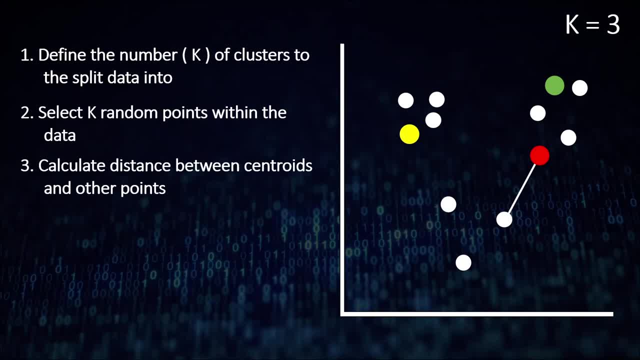 We can then calculate the Euclidean distance between the cluster center point and all other points. If we take this point here, for example, we can see that it is closer to the red cluster compared to the green and yellow clusters. As a result, it gets assigned to the red cluster. 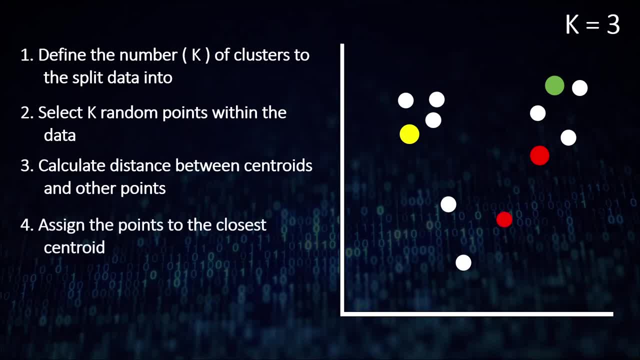 We then repeat this process with all other points on the scatter plot until we get our k-randoma point been assigned to an appropriate cluster. After all the points have been assigned to a cluster, we can then calculate the mean point of each cluster, which are represented here by the x's. 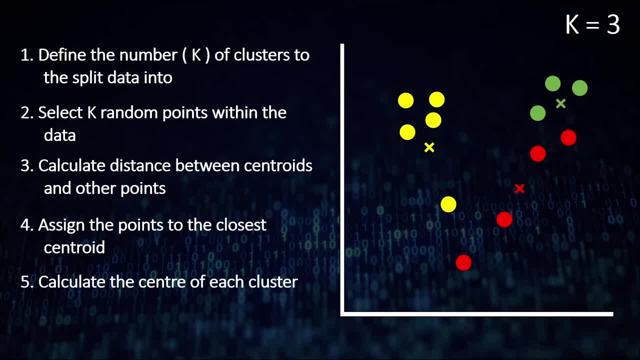 After the new mean points have been calculated, we can then repeat steps 3 to 5 and check if the points belong to the same cluster or to a different one. As we see here, a few points have changed their colour as they are now closer to different. 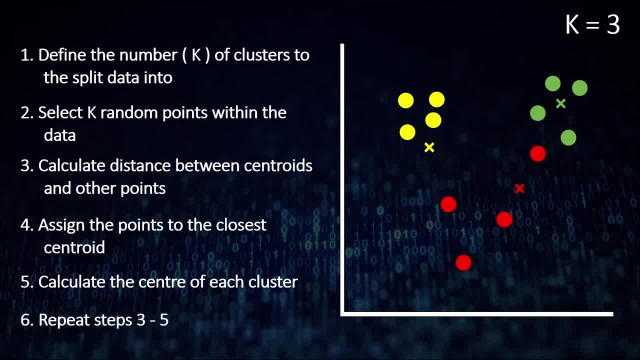 mean points. Once the points have been reassigned, we can then recalculate the mean point and repeat. Eventually we will reach a point where the mean points of the clusters do not change, and then we have our final clusters. And this is just a very simple illustration of how k-means clustering works. 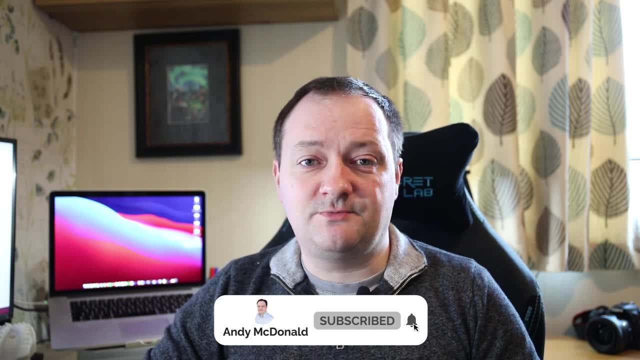 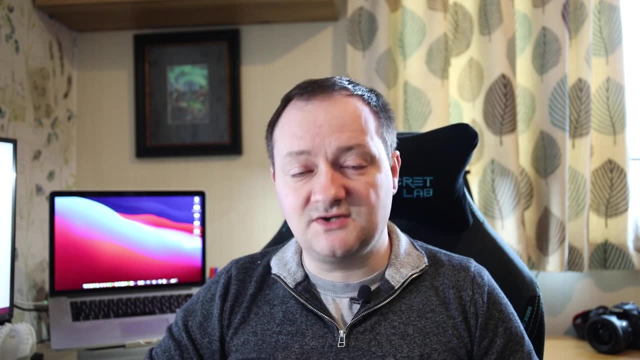 Now that we have the basics of k-means clustering covered, we can now go to our Jupyter notebook and see how we can apply k-means clustering from the sklearn Python library to some well-logged data. So let's go over to our notebook and get started. 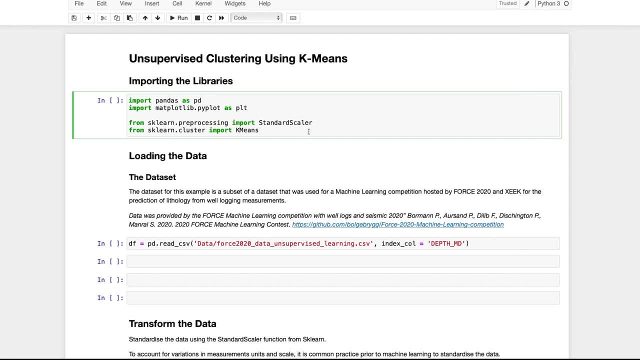 In this tutorial we are going to see how to run a simple k-means clustering on some well-logged data. Don't worry too much if you are not familiar with well-logged data. the same process can be applied to other datasets. 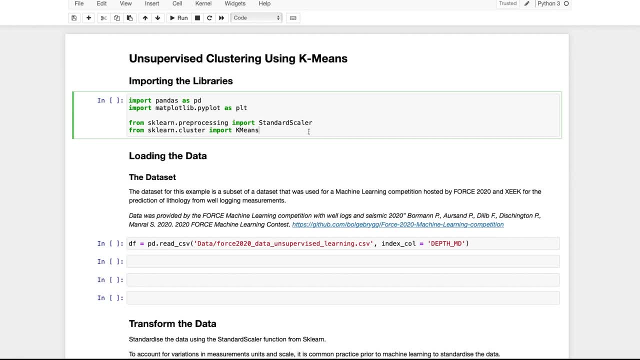 So the first step is to import the main libraries that we are going to be using. We will be using pandas, which is commonly imported as pd, and this will be used to load data from a CSV file and also view our data. We then have our import matplotpyplot as pd. 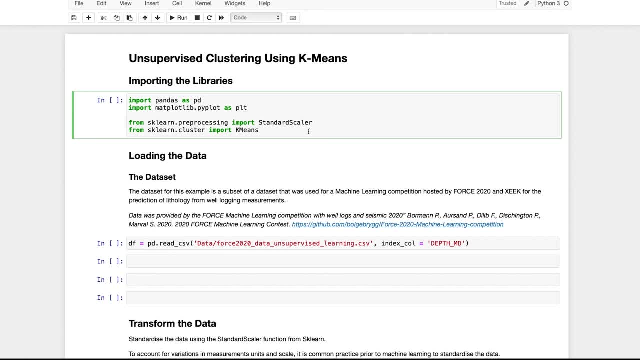 And this is the main plotting library that we are going to be using to display our results. And finally, we have the main library and modules we will be using for our machine learning process. These are the standard scaler from sklearnpreprocessing and k-means from sklearncluster. 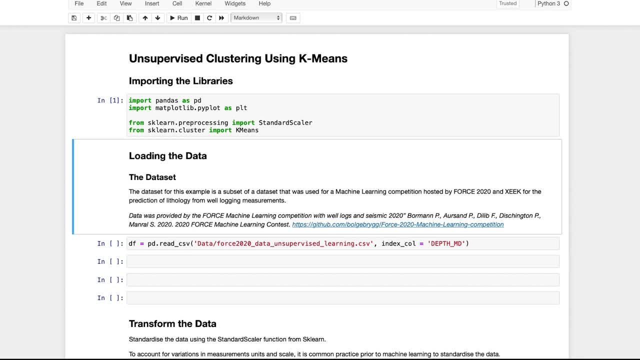 Once our libraries have been imported, we can then move on to loading the data. The data we are using today is a single well from a much larger dataset that was used for a machine learning competition hosted by Zeek and Force 2020.. You can find a link to the full dataset and the competition details in the description. 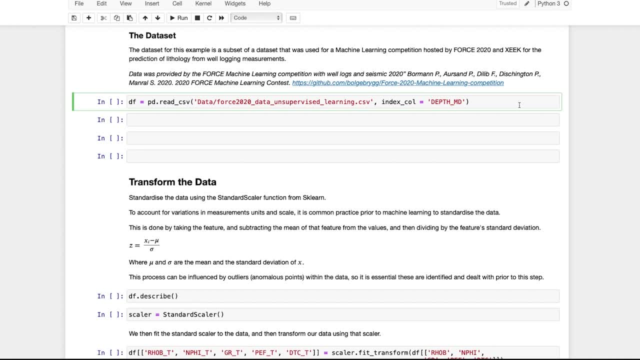 below To load in our data. we will call upon: df is equal to pdread, underscore, csv. and then we pass in the location and the file name. To make things easier for us and to make it easier to work with our data, I am going to 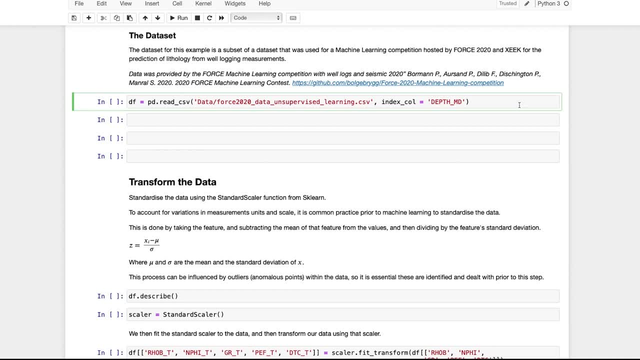 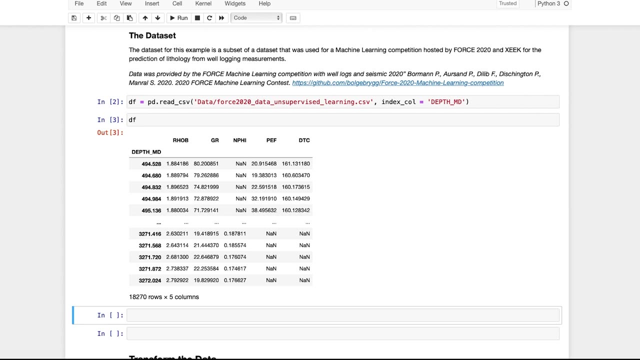 set the index column to depth underscore md, And this is just the measured depth that has been acquired along the wellbore, And once we have run that, we can check our contents by calling upon the dataframe or the DF variable. Then we have our measurements from each of the logging tools. 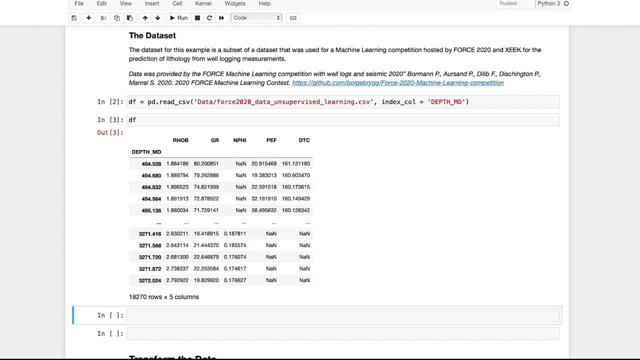 Ourо B, which is the bulk density, Jr, which is gamma ray, nφ, which is the neutral porosity, pθ, which is the photoelectric factor, and DTC, which is acoustic compressional slowness. As you can see from the protobizome, we have a series of NANs within our data. 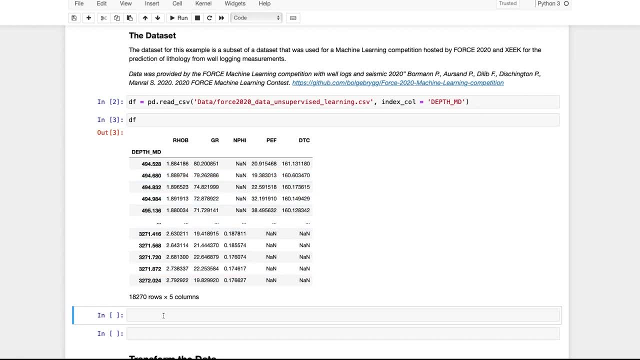 This means not a number or missing values. Many machine learning algorithms can't handle the missing values. pierANS, P et regain reduced minus 1 a-p Estimation. 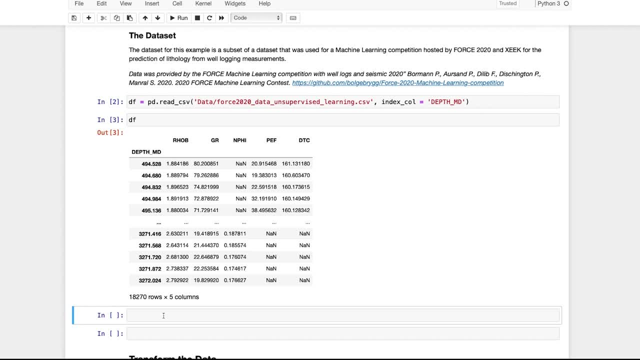 have to either repair them or remove them, and in this situation, what we're going to do is we're going to remove them. and just to keep things simple, I have done a video previously looking at various ways to fill the data using pandas. you can check that out on my channel if you're. 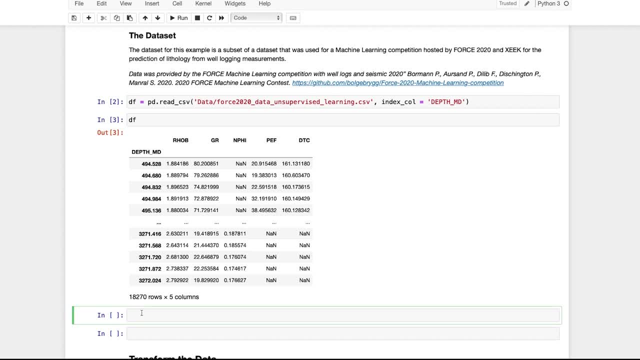 interested. So to drop our missing values, we can call upon dfdropna and in the brackets we'll set, the argument in place is equal to true. So, rather than creating a copy of the data frame, what we're going to do is apply this function dropna to the actual data frame, here and now. if we look at our 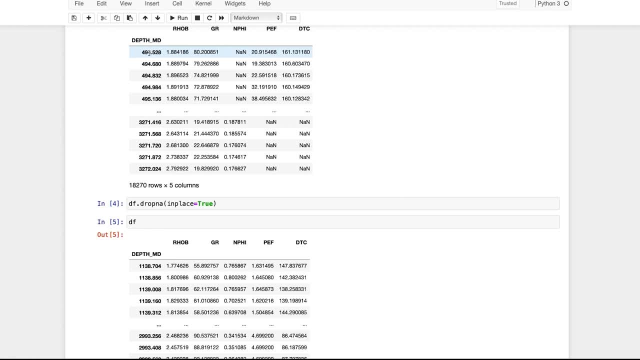 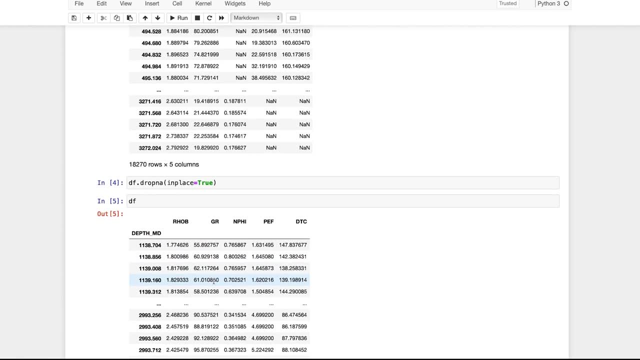 data, we can see that some of the rows have disappeared, so the debt value of 494.528 is now no longer within the data frame and we can see that we don't have any nans within here- and we can further confirm this by calling upon the described method- and we can see that the count 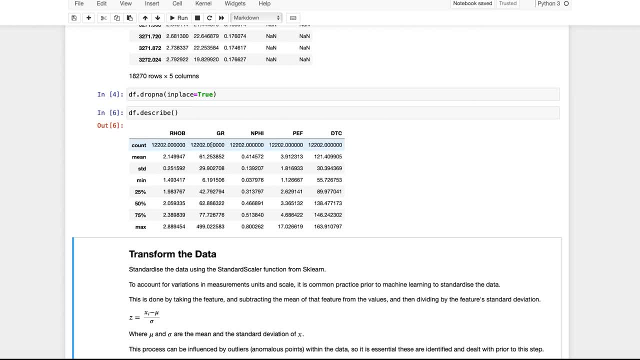 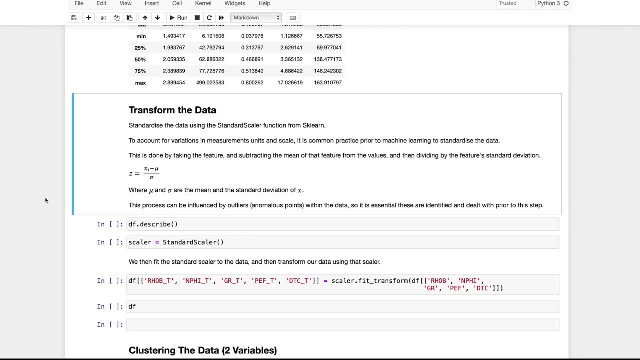 is equal for all of the individual columns within our data frame and this just indicates that there are no values. So we can now apply this function dropna to the actual data frame here and we can see that there are no missing values. So the next step within our process is to transform the data. 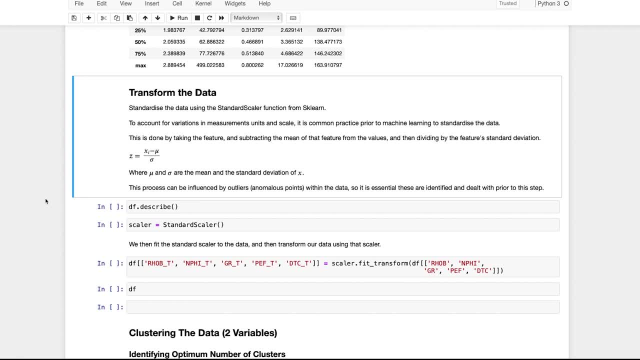 So, before we apply our k-means clustering algorithm, we need to standardize the data, As our data set contains features that have been measured in their own units and have their own data ranges. some features may end up having more influence over the final results compared to. 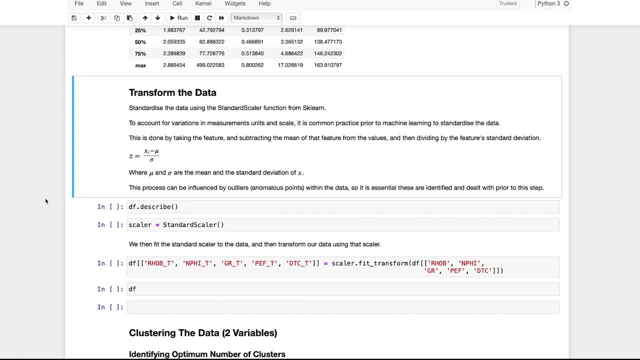 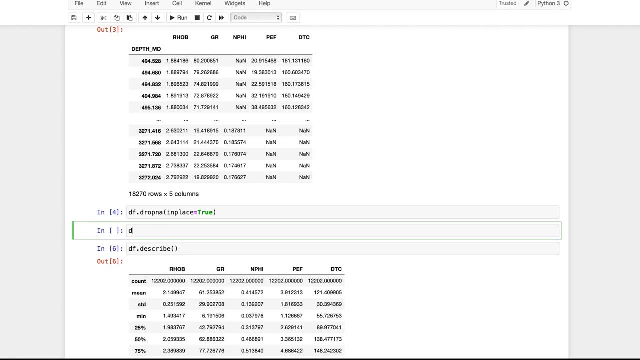 others. To reduce this impact, we need to take each feature, subtract the mean of that feature from each value and then divide it by the feature's standard value. So we can see, for instance, that if I call upon the new data frame here just to get our values, 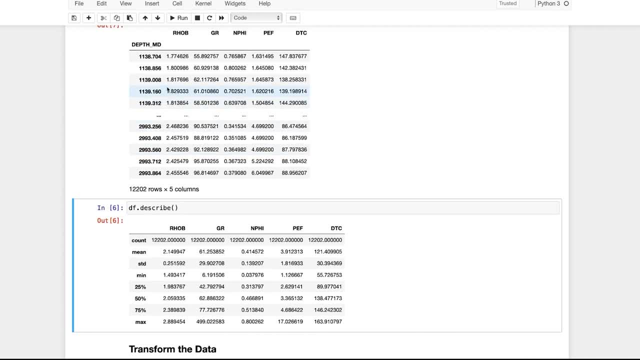 above this dfdescribe method. we can then have a look at the values and how this process works. So we have the first value here within the row B column, which is 1.77, and then we have a mean of 2.1499 and we also have a standard deviation of 0.25.. So what we do is we take 1.77 and take away. the mean from that, and then that result is equal to the standard deviation of 1.75.. So we can then, then we have a standard deviation of 0.25.. So that's the first step within our process are the first thing we need to do is we need to take out the mean from that, and then that result is. 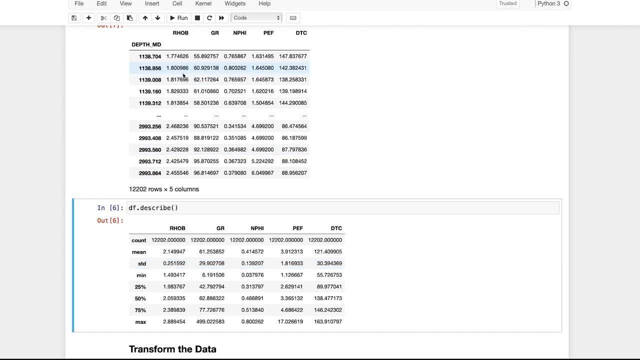 the value of that, and then we need to take out the mean from that, and then that result is the mean from then divided by the standard deviation, and then this is repeated for each of the measurements within this column. Once that's been done, it will then be applied to the other columns within this. 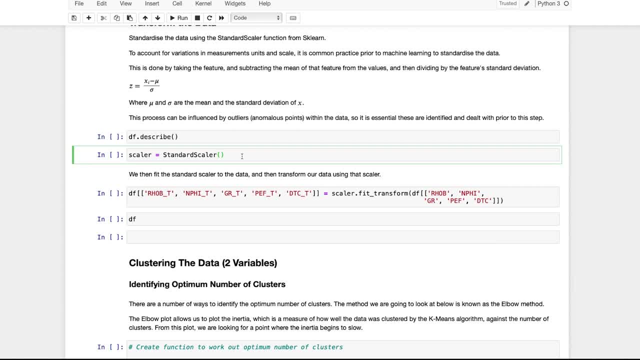 data frame. So let us apply the, the standard scalar. So first we have to create an instance of the scalar and we can do that by typing: scalar is equal to standard scalar, open brackets, and that will initialize the class. So then we need to fit that standard scalar to our data and then transform. 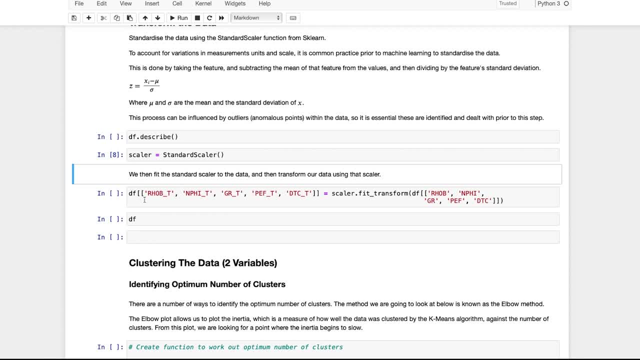 our data using that scalar. What we need to do is within our data frame. I prefer to have those curves or those outputs put back into the data frame rather than having them as an independent array. So what I've done here is I've added the curves with an underscore t to say that they've 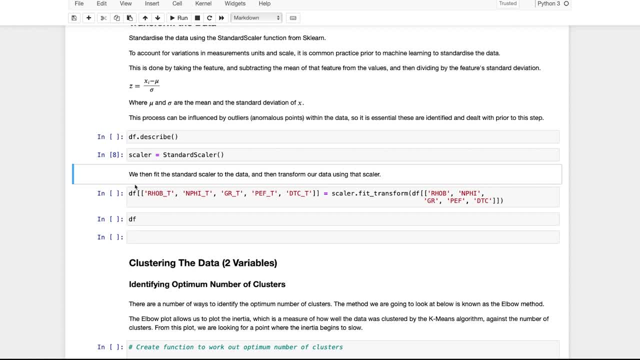 been transformed. Set that up as a list within the data frame object. So this is going to add new curves to our data frame and over on the right hand side. well, we need to call upon scalar and then we call upon this method called fit underscore transform. 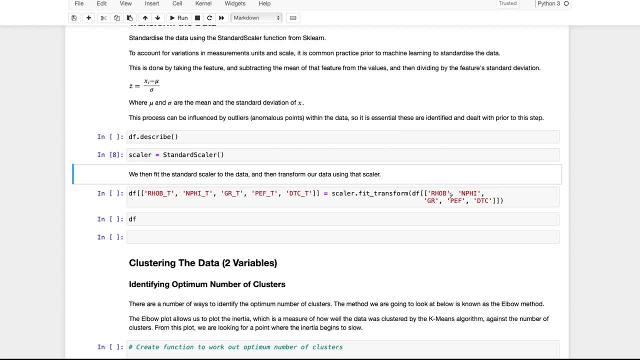 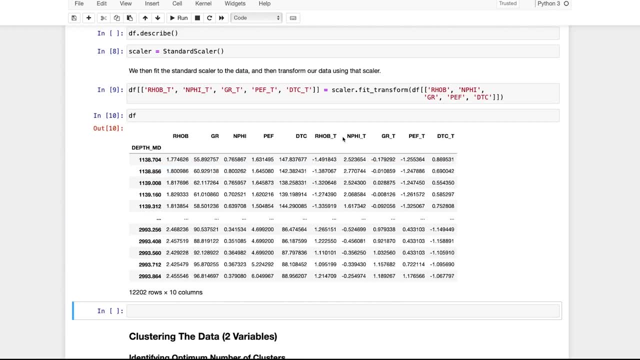 And then we pass in our data frame with our original curves that we want to transform So we can run this. and then, when we view our data frame, we can now see that we've got our row b- underscore t, n, phi, underscore t, etc. here in the data frame and we also have our original values. 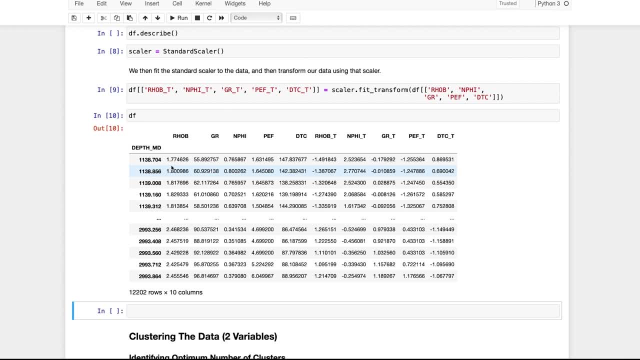 So why am I doing this? Well, it just makes things easier when we come to plotting. So if I had done this without applying it back to the data frame, we would be working with a numpy array. We would then have to work out how to do that. So we're going to do that by applying a numpy array to 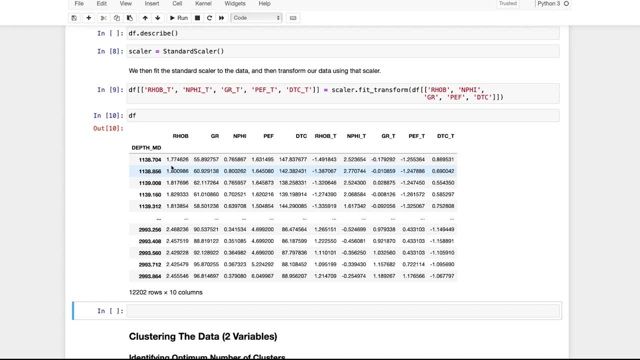 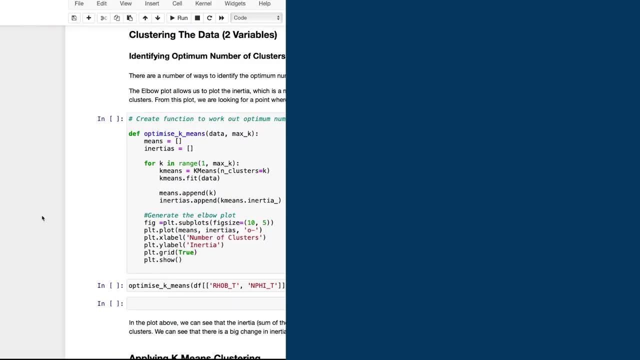 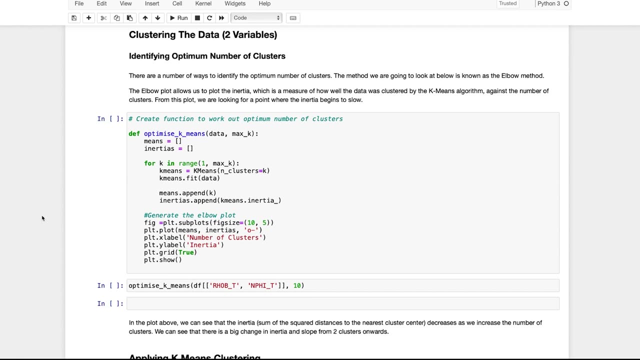 the data frame, which can be done with a few lines of code, but this is probably the. in my opinion, there's the simplest way to do that: to bring it into the data frame. Now we're going to move on to actually applying the k-means clustering to our data. But you may have one important question. 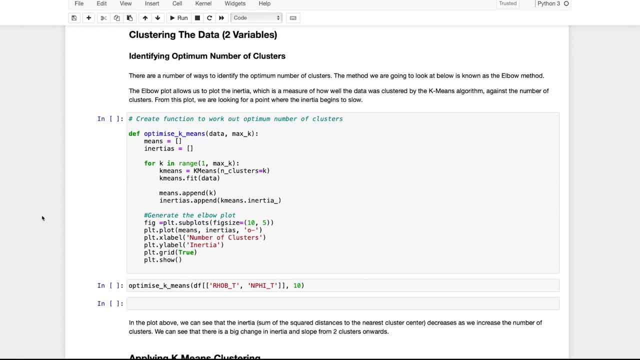 that you're asking, and that is: how do we know how many clusters to initialize our algorithm with? You would have seen in the presentation at the start that we we need to provide a number for k to begin the process, So we're going to do that by applying a numpy array to our data frame. 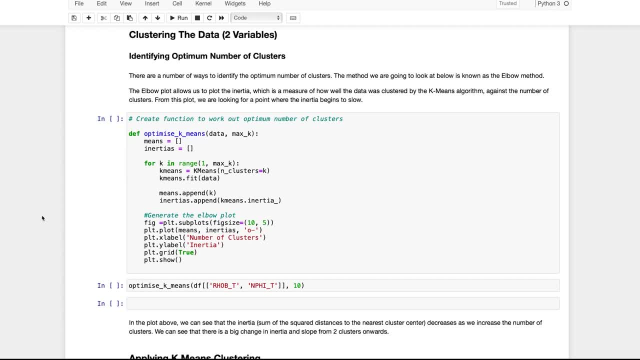 There are a number of methods we can use to identify the optimum number of clusters, and the one that I'm going to show here involves a plot known as an elbow plot, And, to keep things simple for visualization later on, we're just going to work with two variables: n, phi, underscore t and. 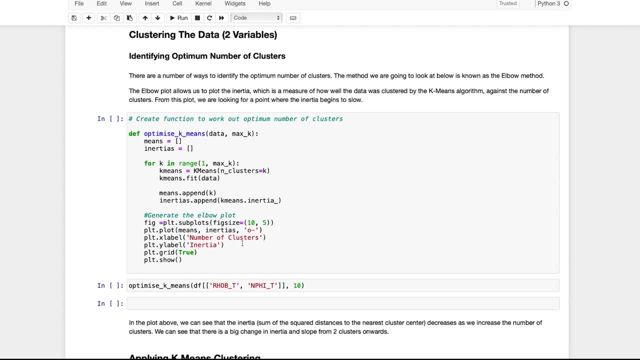 rho b underscore t. So the simple idea behind this function is we run our k-means algorithm multiple times and plot the inertias, which is simply a measure of the sum of the square root distances to the nearest cluster center. As the number of clusters increase, the inertia will. 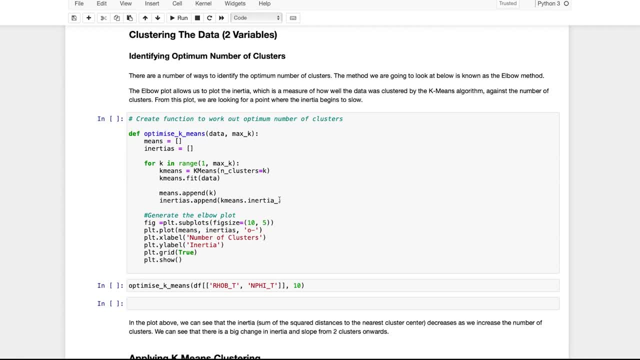 decrease and there will be a point in this plot where the value will go from a large change between clusters to a very small change between clusters. It is at this point that we have an idea of what our best number is for starting our k-means algorithm. So with this function I've got two. 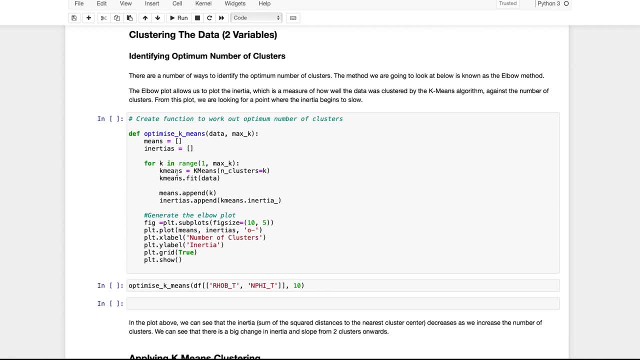 lists that are being created here- means and inertias- and then we're going to look through k, so we're going to range from one to maximum, and then we're going to look through k to maximum, So we can pass in any number here and it will look through that until we've reached the maximum. 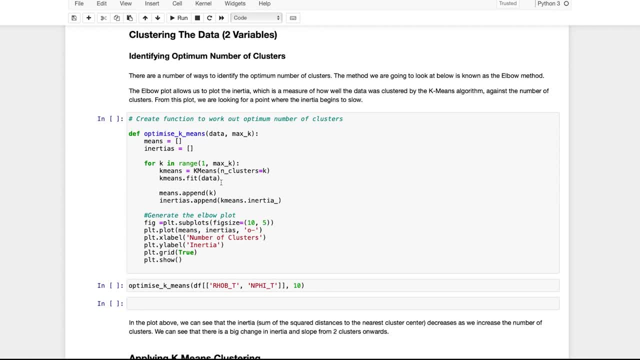 number of k, and then we're going to apply the k-means algorithm and then fit that algorithm to the data, and then we append the inertias to our list as well as the k number to our means list, and then we're just going to generate the elbow plot down here by just creating a simple matplot. 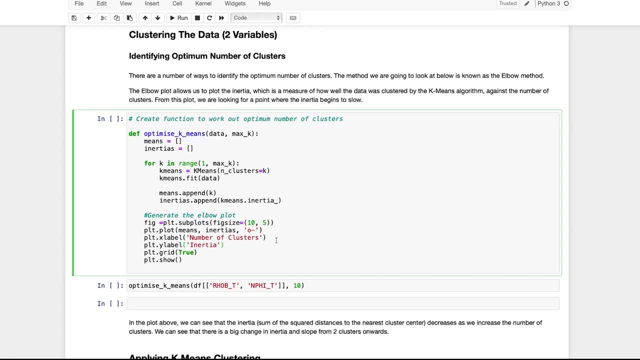 lib figure showing their number of clusters versus inertia. So to keep things simple for visualization, we're just going to work with the two variables n- phi underscore t and row b underscore t, and then we're going to pass in 10 for our maximum number of clusters. So let us run this. 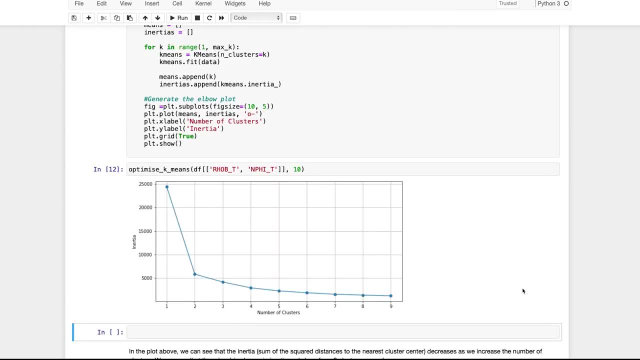 function once it's run. we then get back this elbow plot and we can see that we've got our inertia up here on the y-axis and the number of clusters here on the x-axis. So here we've got cluster one which has a high inertia, which means that the sum of the squared distances between the cluster center 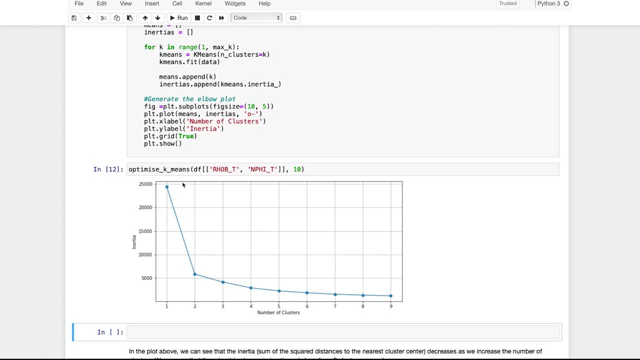 and the points is very, very high As we move into two-dimensional visualization. we're just going to go with two clusters. we then reduce that number for inertia down significantly to around about six thousand and then, as you can see, we've got a now. we've now got a gradual decline in our inertia. 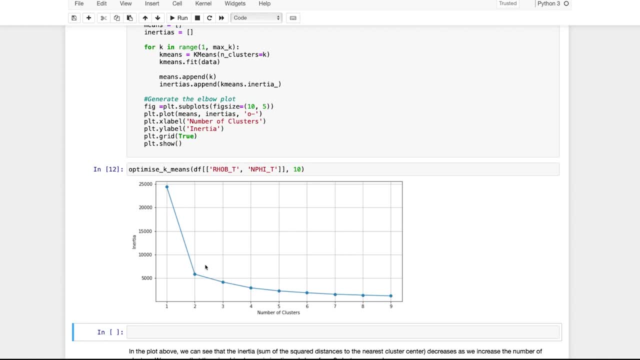 as we move along. We could select our point here at two clusters, or we could potentially select three clusters, as that slope is getting more and more gradual as we go above three clusters. So two clusters might be just a bit simplistic for this kind of data, so I'm going to go with three clusters. 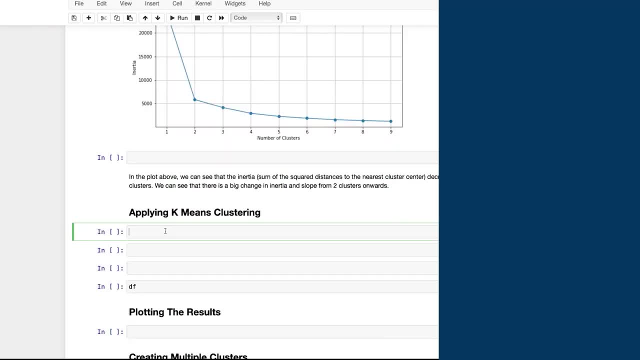 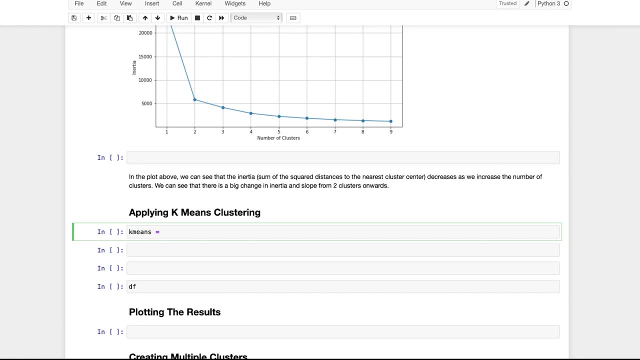 for this, this data set. So, now that we have our initial value for k, we can then create a new variable called k-means, and that is going to be equal to k-means, which is our algorithm that we've imported from sklearn. and then we're going to set the n, so the number of clusters, or n clusters. 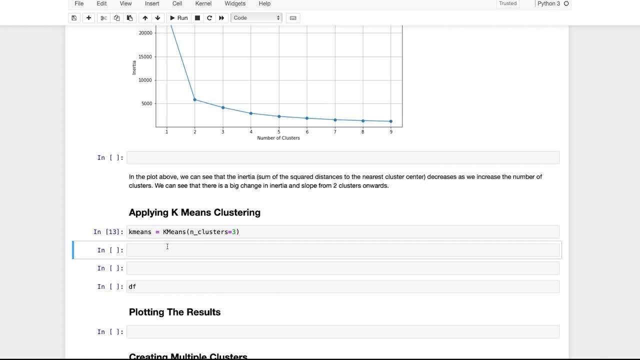 is equal to three. So now that we've initialized our k-means clustering algorithm and we've set the k- the number of clusters- or the k value- to three, we now need to apply the k-means clustering algorithm to our data, and we can do that by calling upon k-means dot fit, and then we're going. 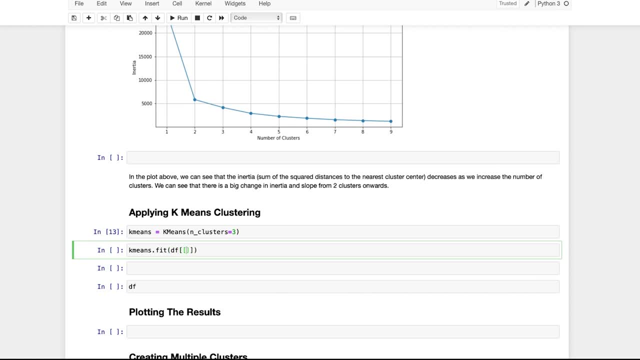 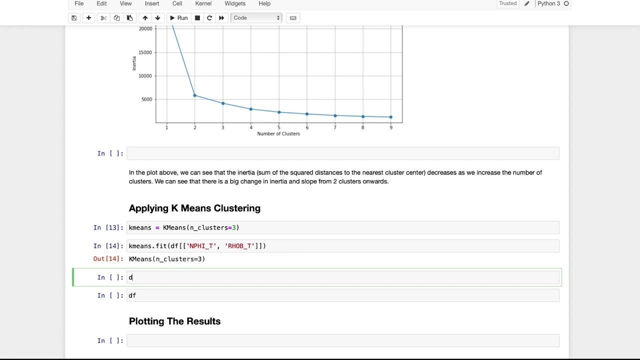 to pass in the data frame and then from that we're going to select our two curves, which will be n phi underscore t and row b underscore t. So that is the k-means algorithm fitted to our data. Let's view the output of this and what we can do is we can just create a new column within our data frame. 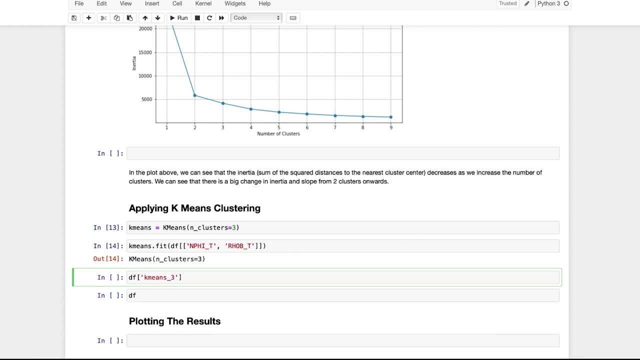 and we will call this k-means underscore free and we will set that Equal to k-means dot labels and we need to add the underscore at the end here and then, when we view our data frame, we now see that we've got k-means underscore free in our data frame and we 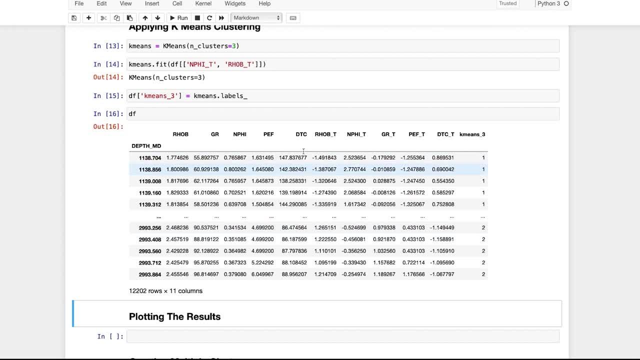 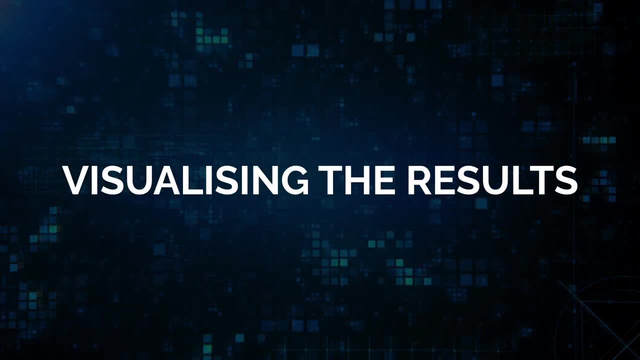 can also see that we've got different numbers here. so we've got a number one for these data points up here and we've also got a number two for these data points down here at the bottom of the data frame. It's all good and well knowing that we've got the data within our data frame as a. 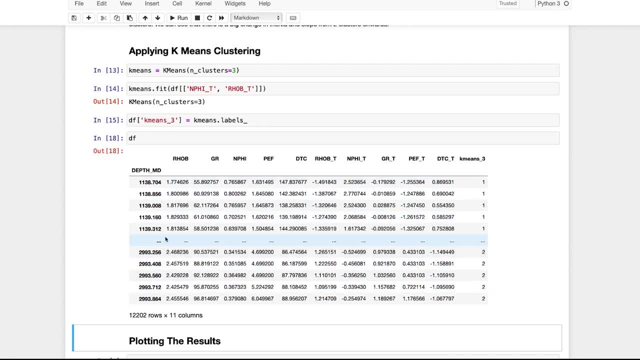 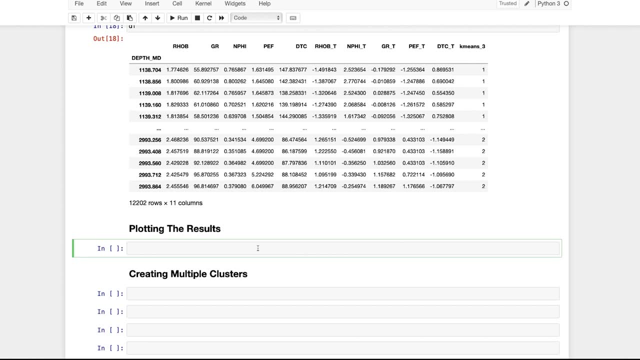 column, but it doesn't really tell as much about our data just by looking at these raw values. So what we need to do is actually plot the results, and we're going to display a scatter plot of our density neutron data, and we can do that by simply calling upon plt, dot scatter, and then we add an: x is equal to df. 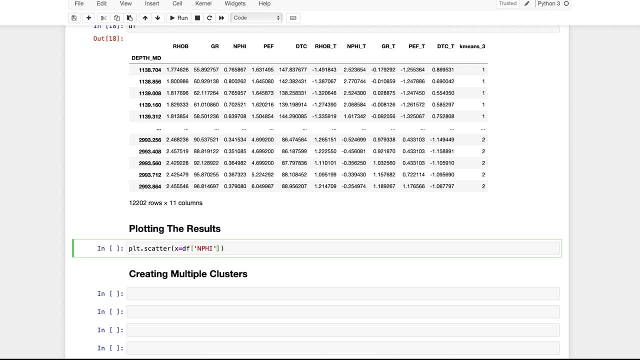 n phi. so we'll have our n phi curve on the x-axis and then we have the y-axis, which is going to be equal to df, and that will be row b. We will also set the color argument c to equal to our new k-means column and we just call upon df. 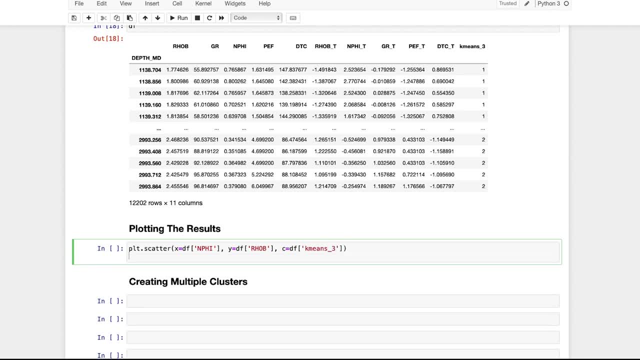 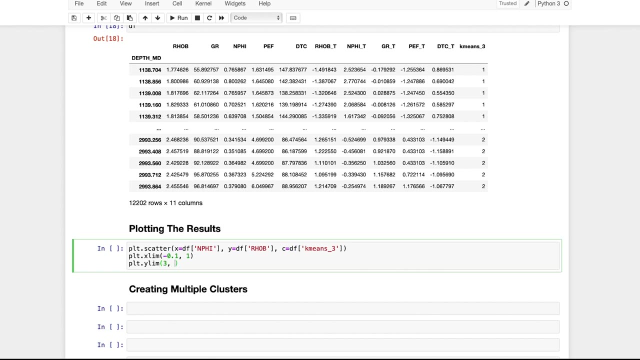 and then pass in k-means underscore free For tidying up our plot. we can then set up the x limits, and we will set that from minus 0.1 to 1 and plt dot y-limb to go from 3 to 1.5. 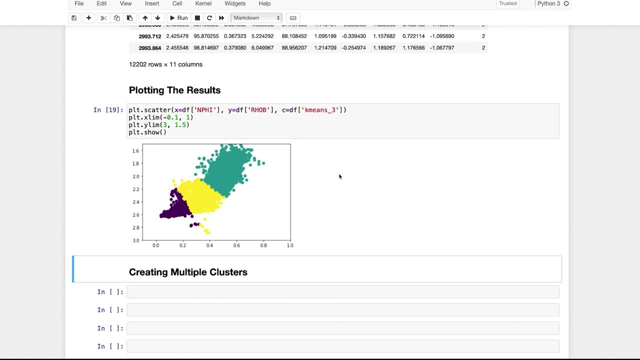 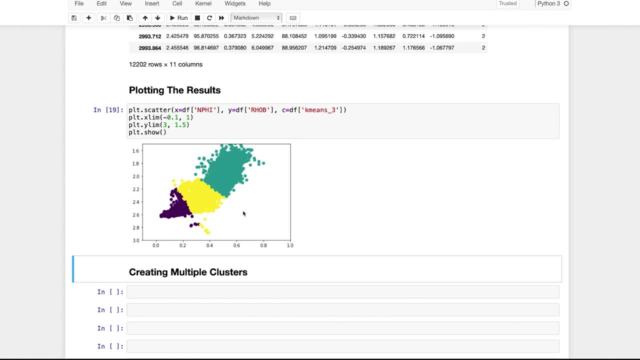 And then we have our density neutron cross plot divided up into different clusters and we can see that we've got one cluster down here in the bottom left and then we've got one in the middle, and then we've got another cluster up here in the top right. 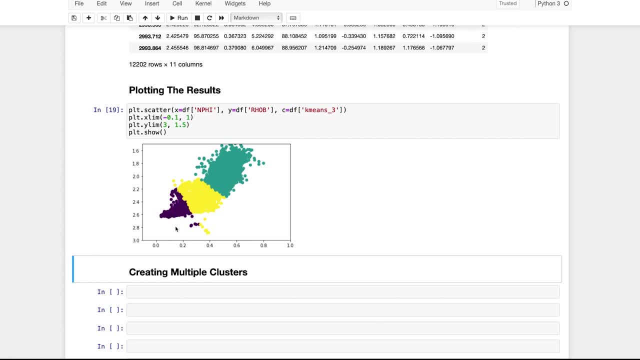 So if you're familiar with reading these density neutron cross plots, we generally have our cleaner intervals down here towards the matrix points of 2.65 for our sandstone or 2.71 for limestone, And then as we move up here towards the right, we get into the shalier intervals and same with up here. 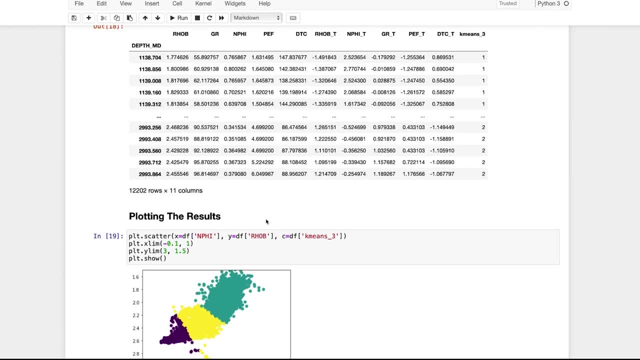 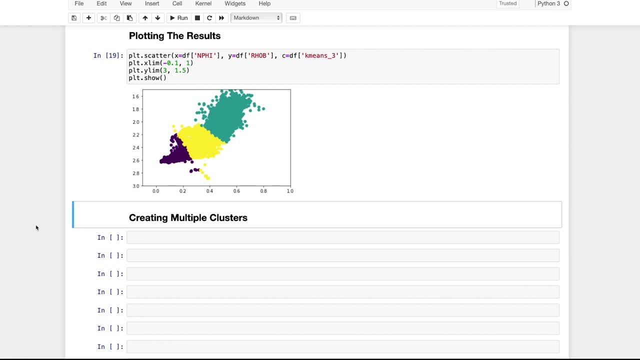 Which could also be from shallower intervals, as we've got quite a large range of data going from shallow to deep. Just for a bit of fun, if we want to see how the k-means clustering algorithm splits this data up using different k values, we can simply create a little for loop, so we'll go for k in range. 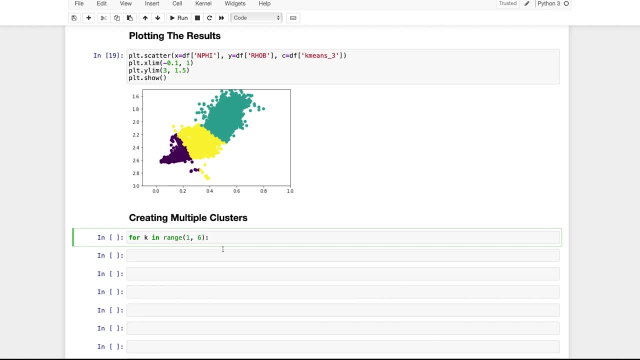 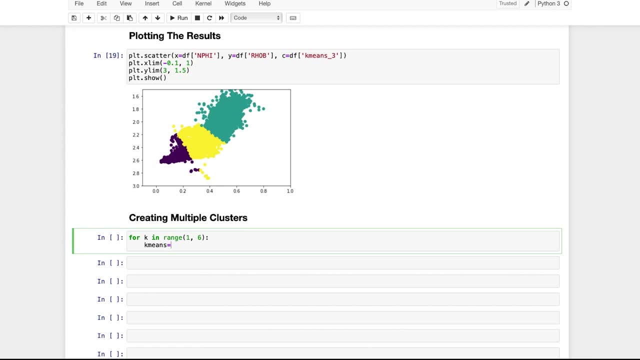 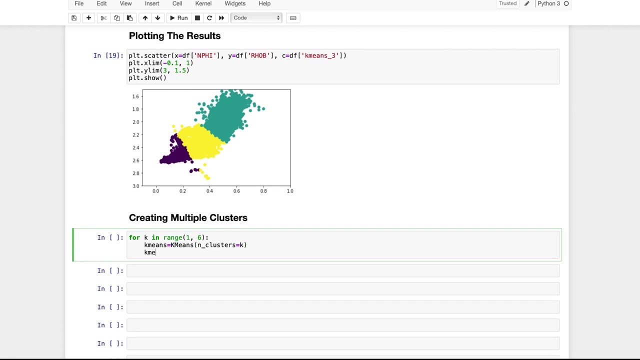 So we're going to go between 1 and 6 and then what we're going to do is run the k-means algorithm- again so similar to our optimization Function- and we're going to set that to k-means and we'll set n. underscore clusters is equal to k and we just need to change that back to a capital, M, and then we'll do k-means dot fit and then we pass in our data frame and also our transform data. 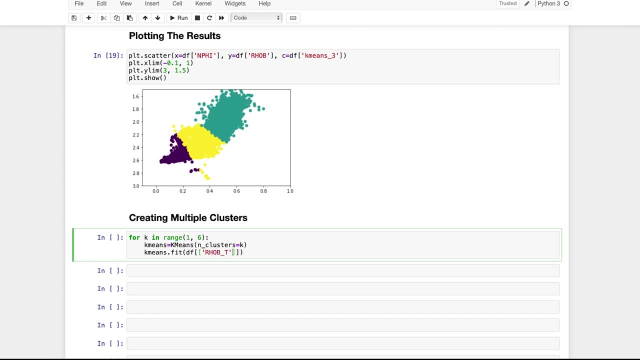 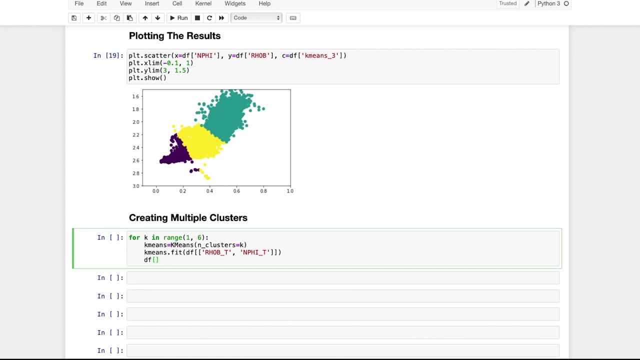 So we'll call upon ruby underscore t and n phi underscore t, And then we will add our new curves back to the data frame and we'll need to create a formatted string by just putting an F at the start and we type in k-means underscore and then the curly braces followed by the single quote. 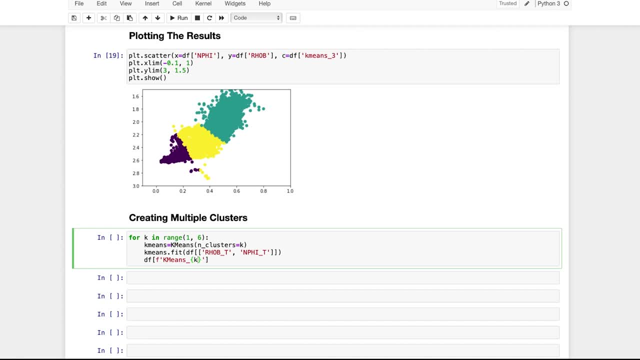 And within the curly braces we can then pass in the k number so that we automatically add a new new column to the data frame with the incremental number or the number representing the number of clusters, And we will set that to k-means. dot labels- underscore. 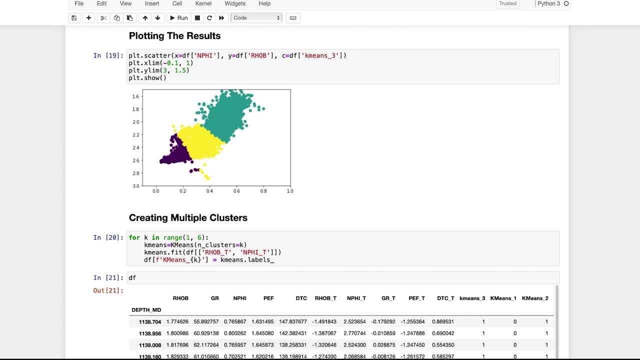 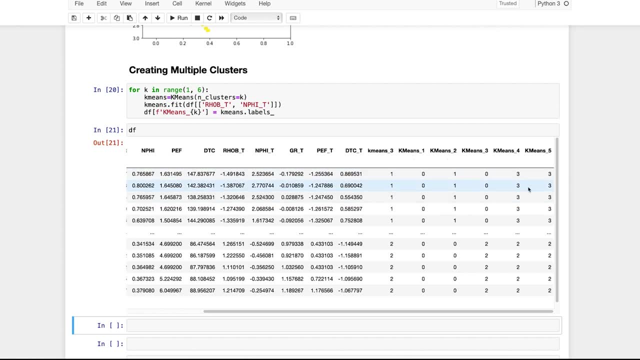 So that's that being done. so if we call upon our data frame now, We can now see that we've got k-means underscore 3 from our original one, and then we've got k-means underscore 1,, 2,, 3,, 4 and 5.. 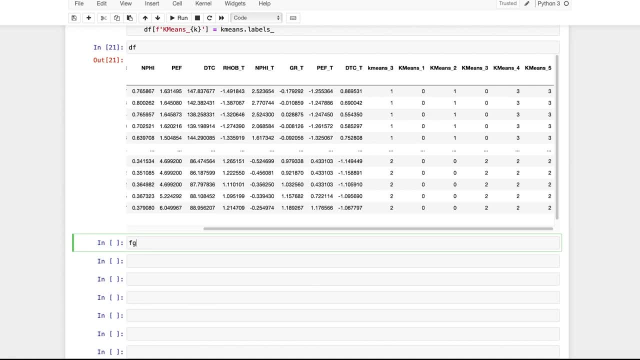 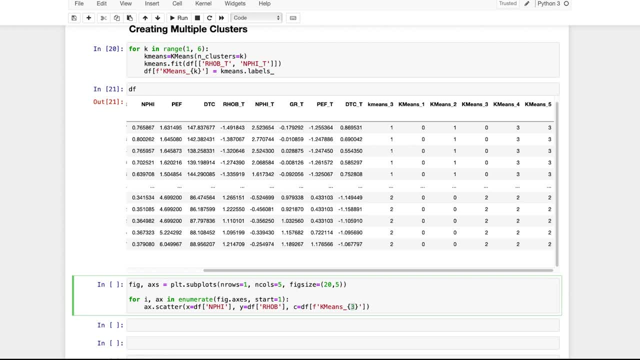 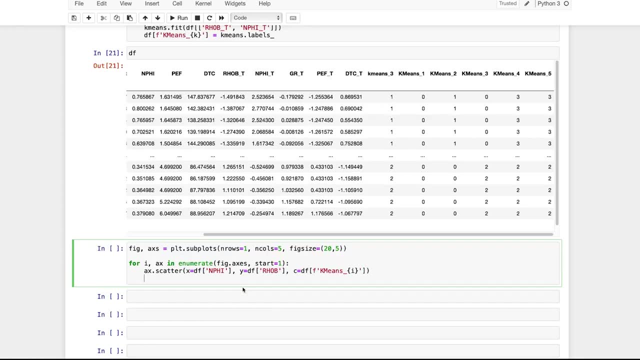 And rows is equal to plt, dot subplots, and then here we need to put in the curly braces and we will use a value of I, so that is going to get the number from the current loop. so, as we're using axe rather than PLT, we need to change the syntax slightly, so axsetYLim. 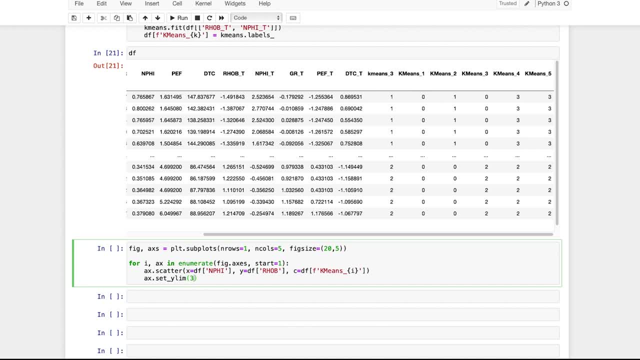 and then we pass in the values of 3 to 1.5 and then axsetXLim, and going from 0 to 1, and then we'll set the title, axset, underscore, title, and then again we use a formatted string, so F, and then open quotes, n, clusters, colon and. 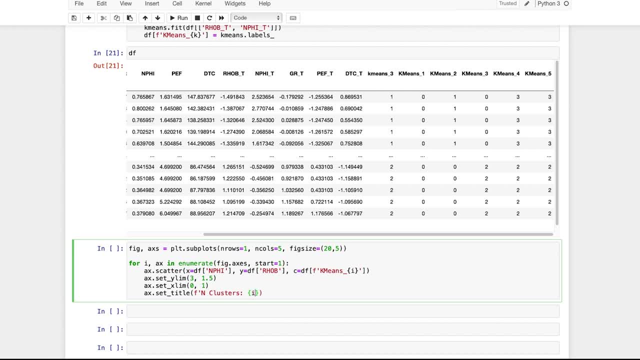 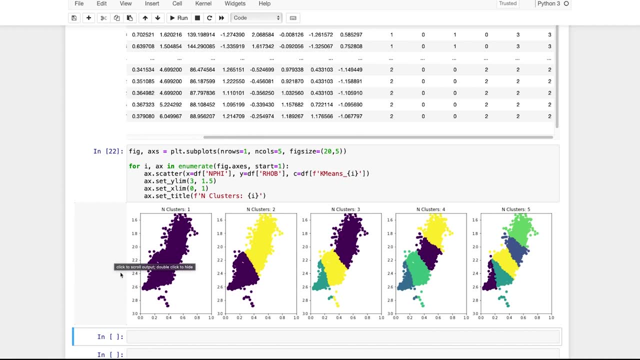 then we pass in our curly braces with the value for I and then we just close that out and here we have our final subplots with the n clusters going from 1 up to 5- see going from one cluster, but where everything is just the same, which we 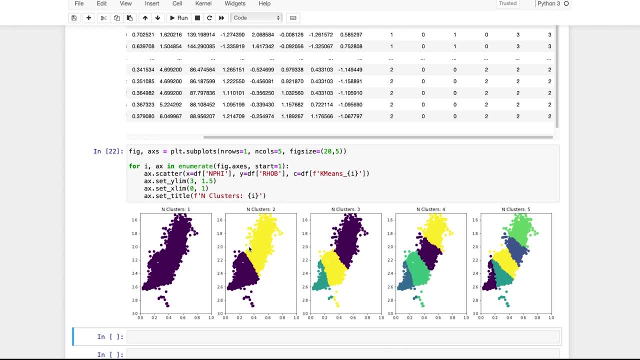 would expect with one cluster and then as we go up to n, clusters is equal to 2. we can then see we've got a single division between the cleaner interval down here and our shalier data up here, and the clusters become smaller and smaller as we go along, as the number of clusters increases. so this is where it. 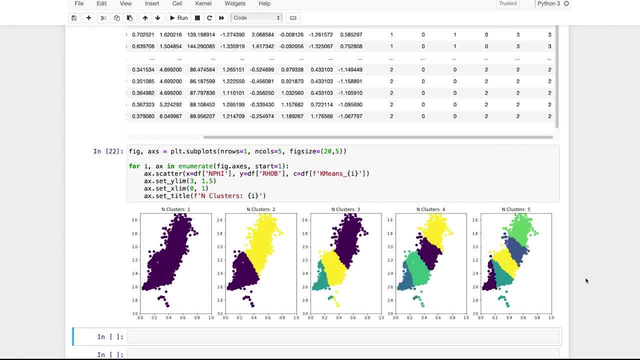 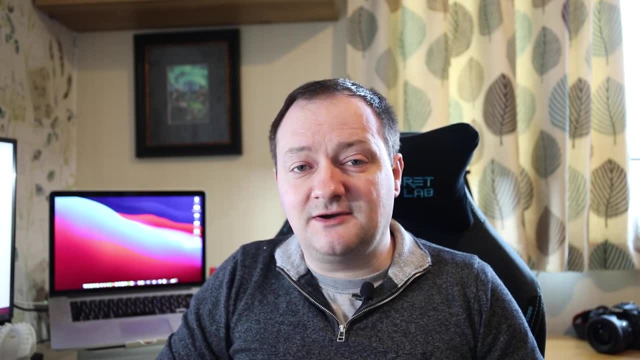 would take some domain expert knowledge to understand whether the k-means clustering algorithm has been applied correctly. so this was just one example of k-means clustering algorithm. so this was just one example of k-means clustering, but there are a number of other different methods and you can see. 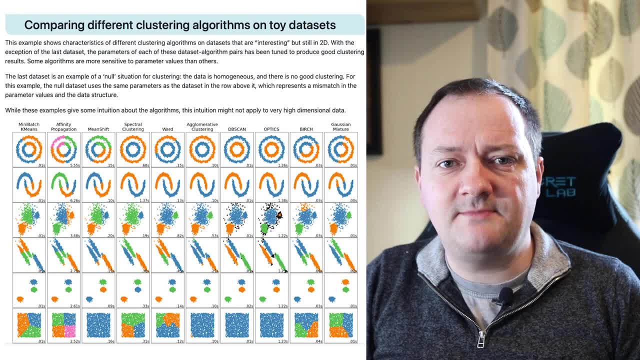 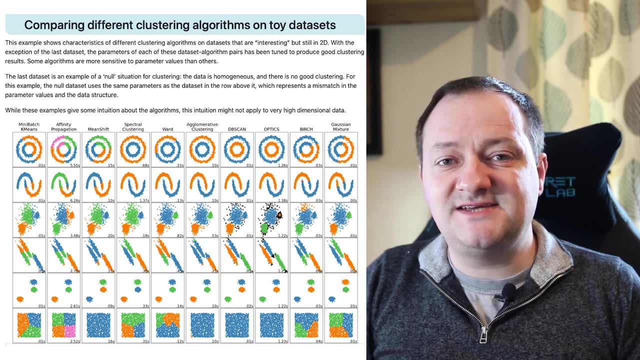 examples of these on the SK learn or the scikit-learn website and you can see here we've got Gaussian mixture modeling, we've got db scan and we've got many other different methods and you can see from this image here how each of these methods split up that data. so instead of importing k-means we can import one of.